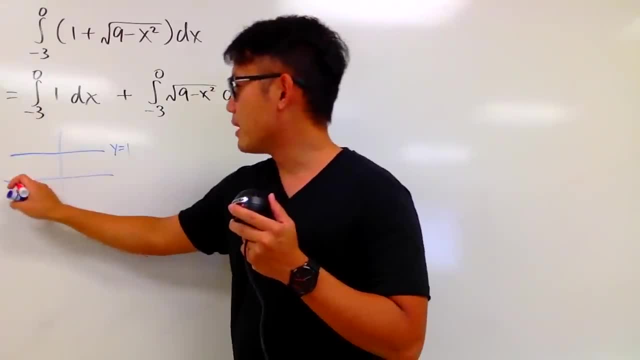 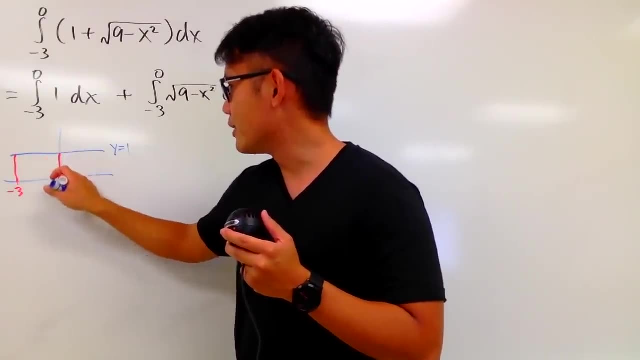 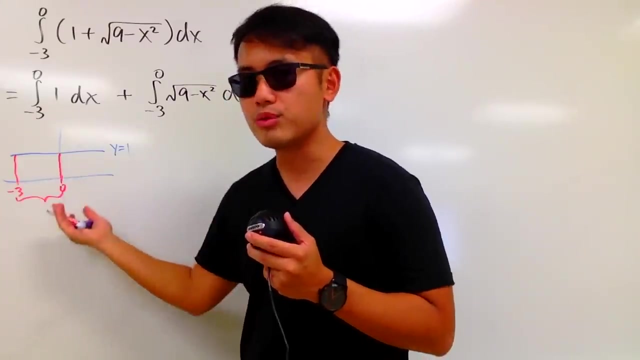 function here. So it's just a straight line and we are talking about from negative 3 to 0, and, of course, this region that we have. it's just a rectangle, And if you look at the base here- from 0 to negative 3, or negative 3 to 0,, look at the distance-wise, you get 3, and then this distance. 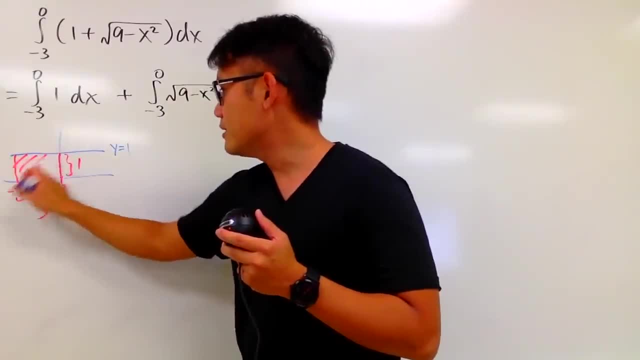 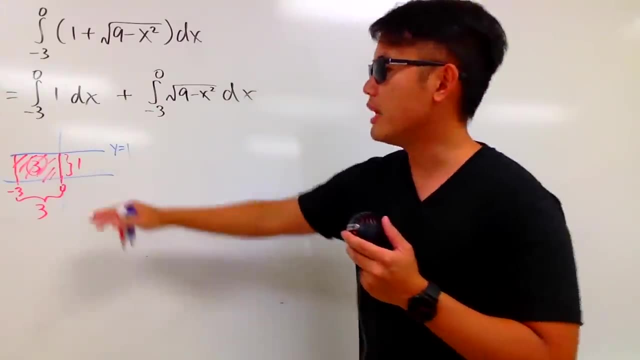 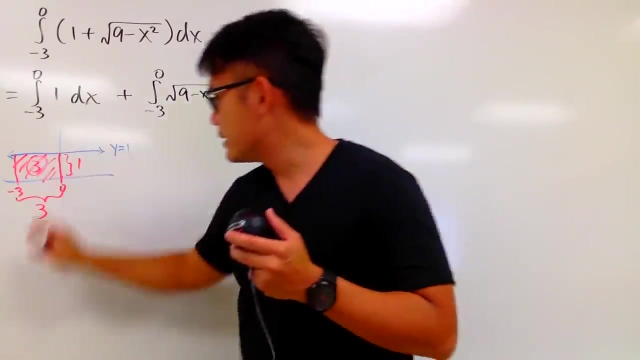 is, of course, just 1.. So to find this area is nothing but just 3 times 1, which is 3.. And it's positive 3 because we are above the x-axis. So this is pretty much it for that one, And I will write this down first This: 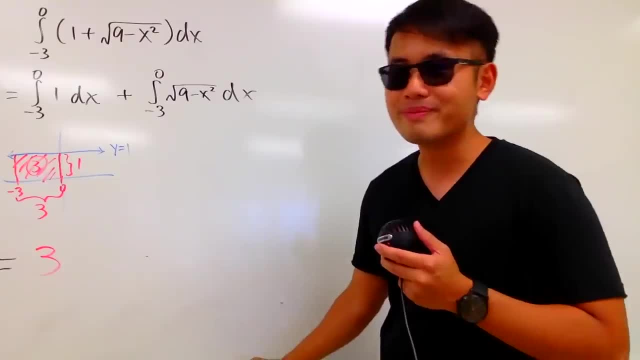 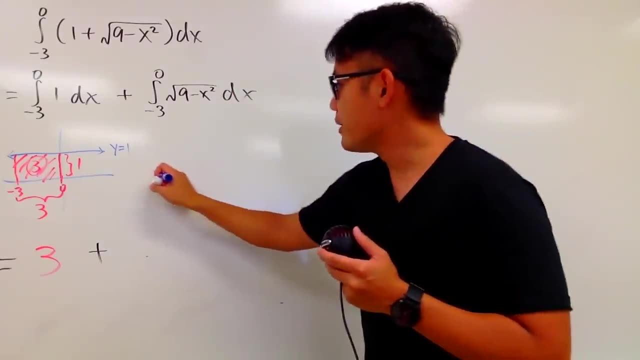 is equal to 3 for the first integral, and we just have to add it with this 1, and we also interpret this as area Right here the graph was square root of 1, and we just have to add it with this 1,. and we also interpret this as area Right here. the graph was square root of 1, and we just have to add it with this 1, and we also interpret this as area Right here. the graph was square root of 1,. 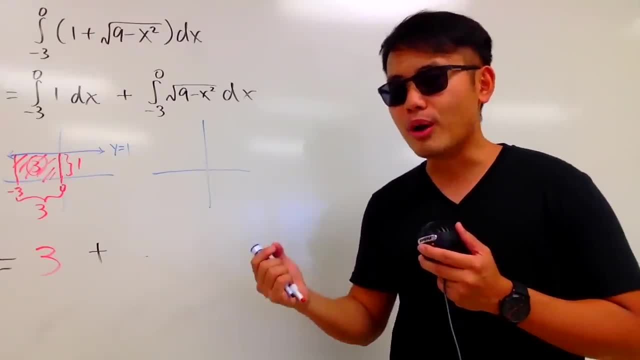 and we also interpret this as area. Right here, the graph was square root of 1, and we just have to add it with this 1, and we also interpret this as area. It's actually a circle centered at 0 and the 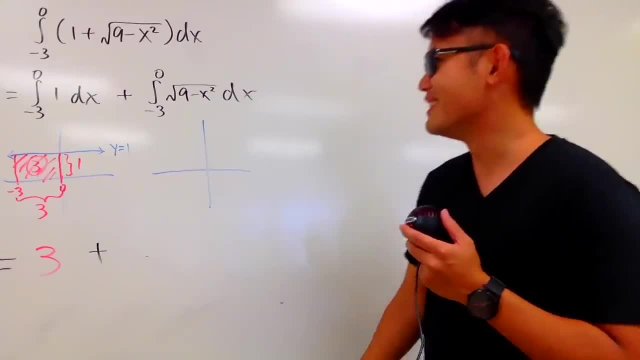 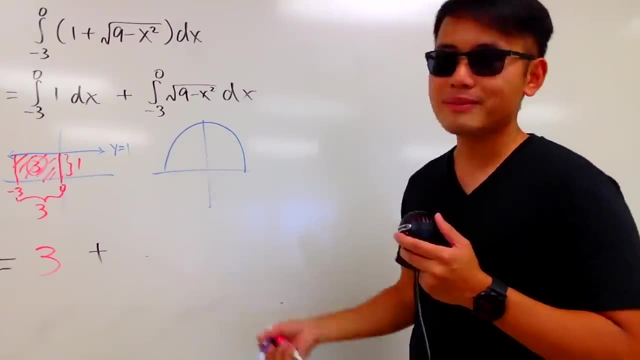 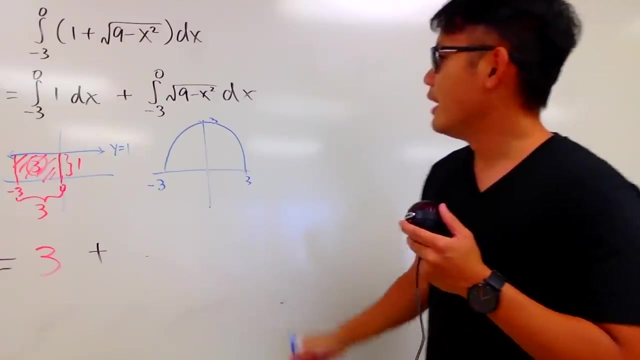 radius is 3, and it's actually just the upper part, because we only have the positive square root. So let me draw this for you guys. first, Let's say: this is my circle, okay, And here is negative 3, and here is negative 3, and here is positive 3, and this is 3.. And to see why this is a circle, 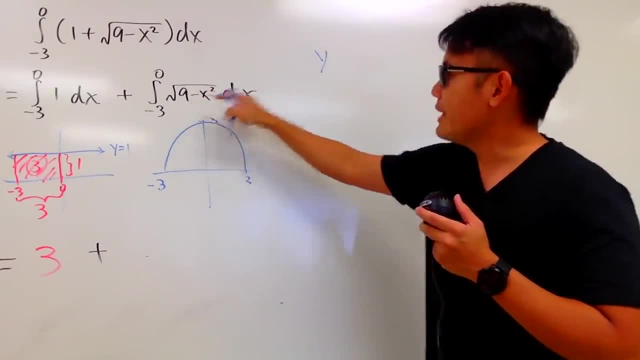 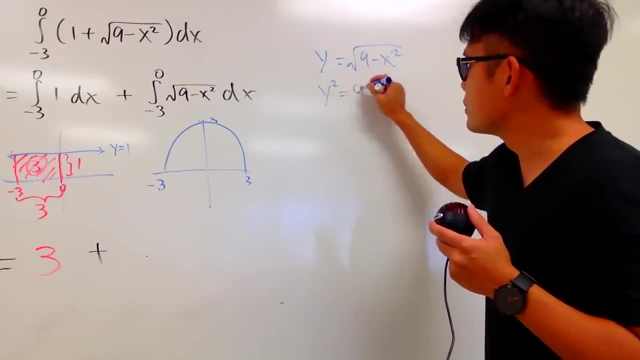 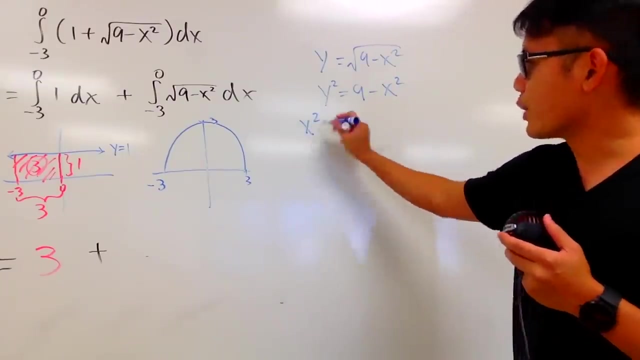 I can just put this down on here for you guys: If you look at y equals to square root of 1, root of 9 minus x squared. We can square both sides so we get y squared equals to 9 minus x squared And then bring the minus x squared to the other side. it becomes positive x squared. 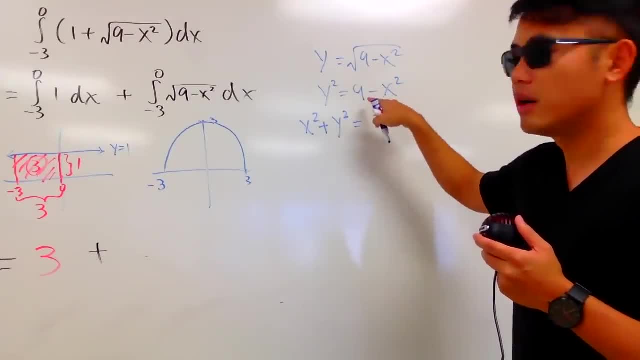 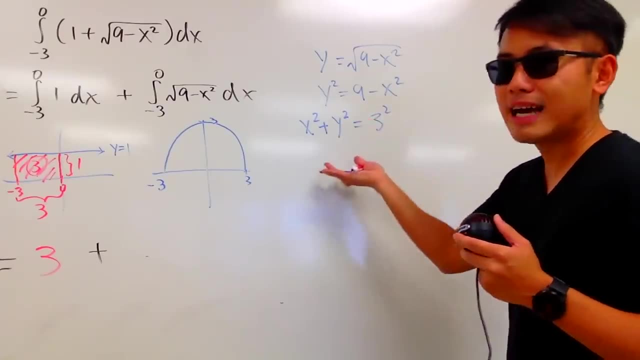 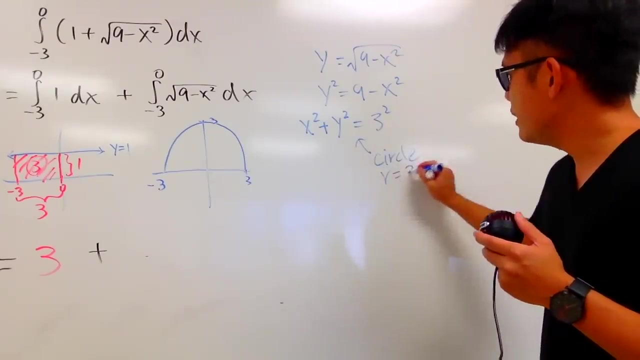 and you add it with y squared and this is equal to 9,, which is the same as saying 3 squared. And if you look at this equation, you should recognize that this is an equation of a circle and the radius is 3, and the center is precisely at 0, 0, because you don't add.